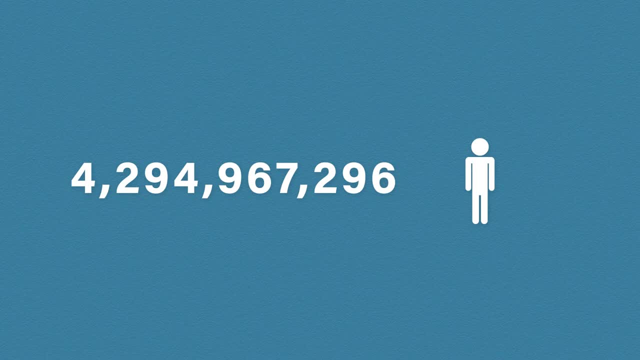 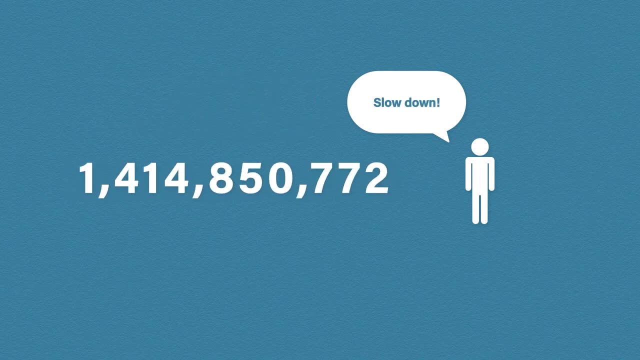 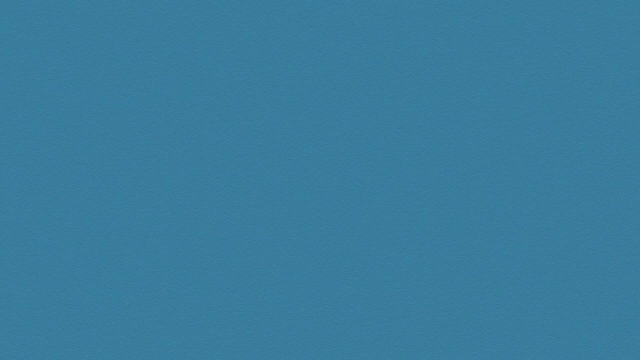 of devices that would require an IP address. If you think about every device you own, like a PC, laptop, smartphone, TV, etc. it quickly became apparent that we would soon run out of IP version 4 addresses. The solution is to eventually move over to the new IP version 6.. 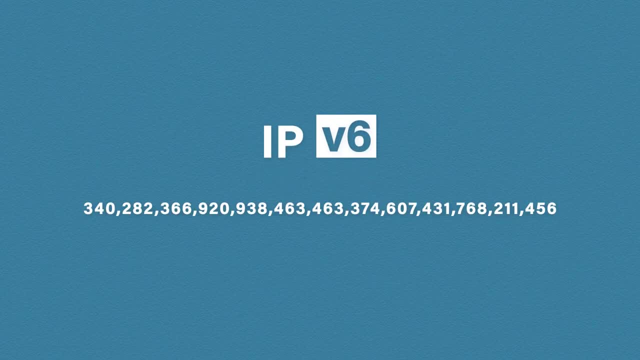 IP version 6 provides us with IP version 5.0.. Well, I'm not even going to try and say that number, but it's a lot. Aside from the number of addresses, IP version 6 also brings a lot of other improvements. 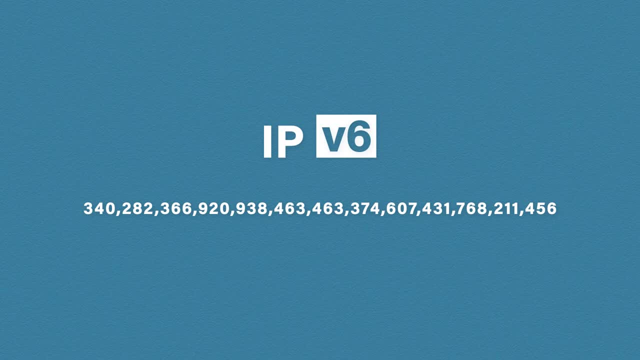 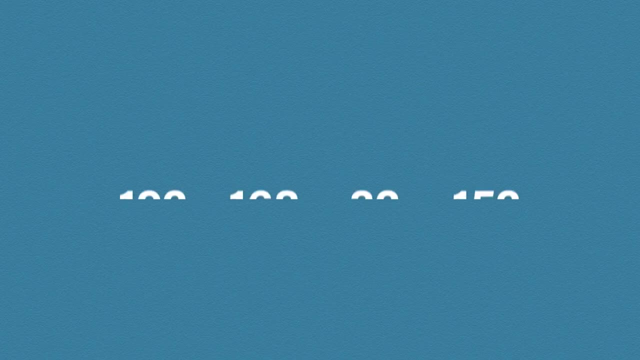 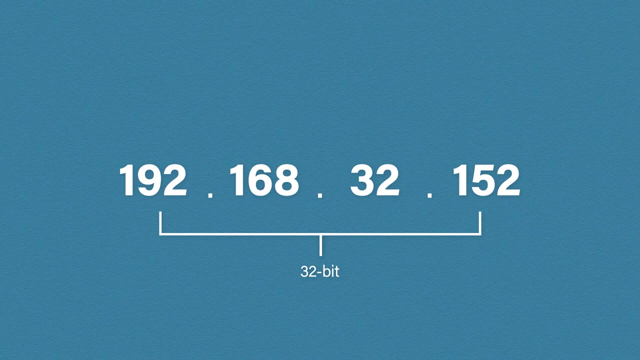 That makes it a lot more efficient and practical. Okay, so let's dive into what an IP version 6 address looks like. Let's first remind ourselves of IP version 4.0. It's 32 bits in length, Remember. bits refer to the binary digits of the address. 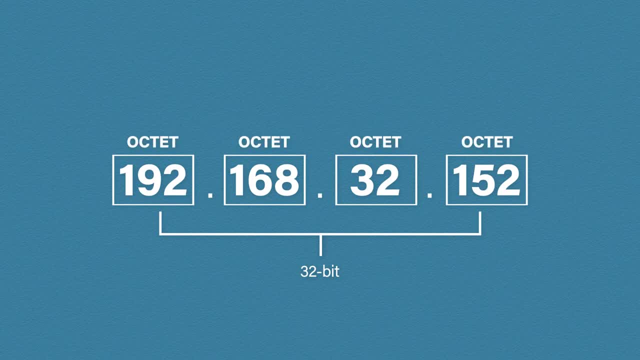 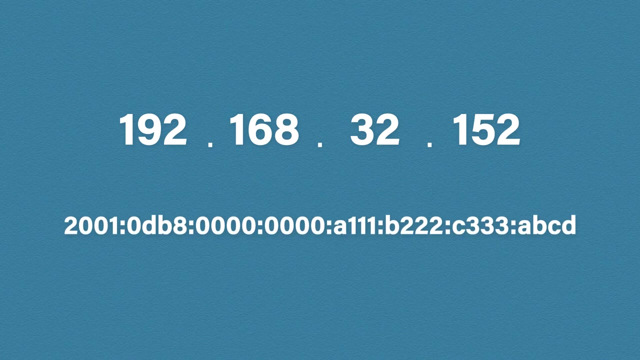 It contains four sections called octets, which are separated by dots, and in theory each octet can contain any number between 0 and 255.. Now we're familiar with our good old friend IP version 4.0. let's bring in an IP version 6 address Now. at first this address looks pretty scary, But don't. 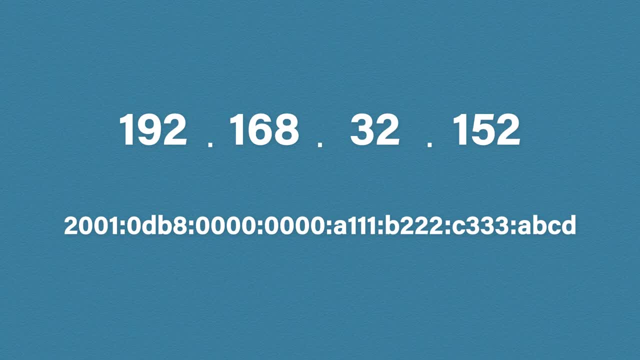 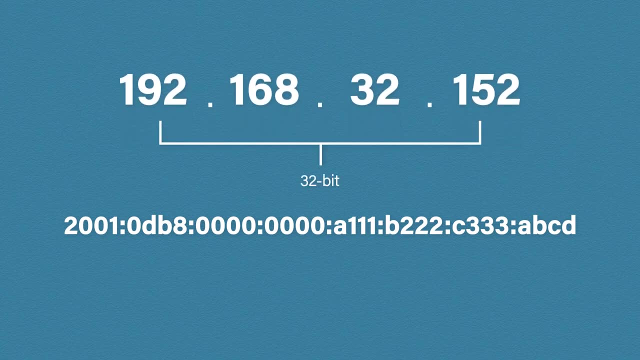 worry, we're going to break it down step by step. First let's do some comparisons. We know our IP version 4 address is an IP version 5.0 address. version 4 address is 32 bits long, but our IP version 6 address is 128 bits. 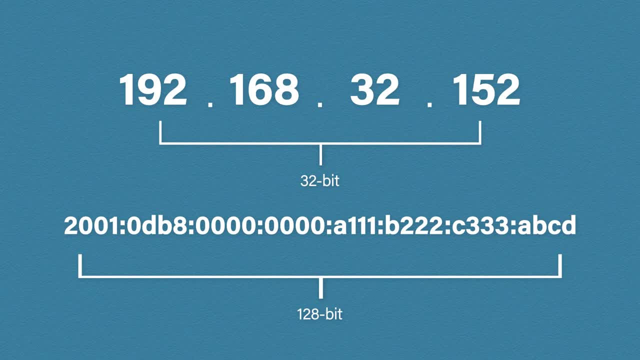 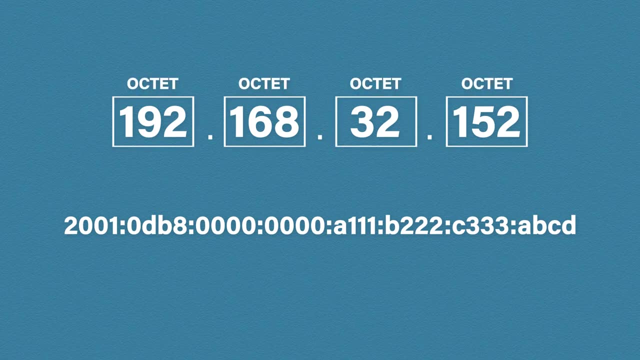 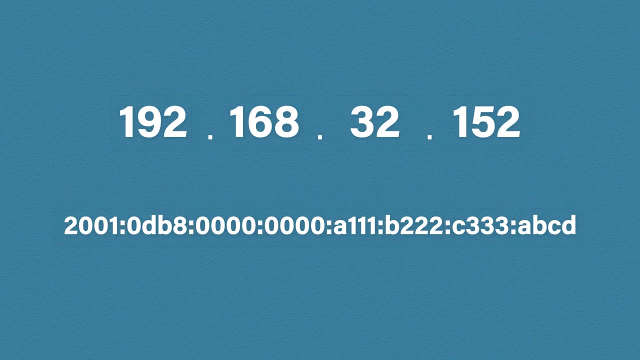 long. This is where we get our massive IP address space from. IP version 4 has four sections called octets. IP version 6 has eight sections, but these are commonly called hextets. IP version 4 uses dots to separate octets, but IP version 6 uses. 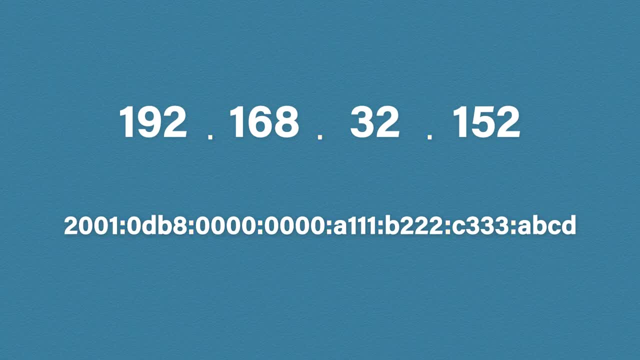 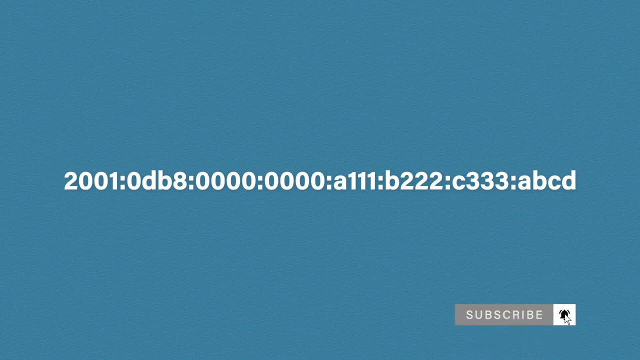 colons to separate hextets. So let's get rid of our IPv4 address and go into some more detail. The first thing you probably noticed is there are letters in this IP address. IP version 6 is hexadecimal, meaning each character can be between 0 and 9 or A and F. 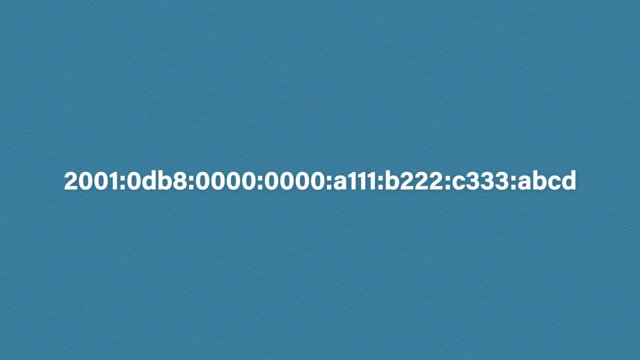 Let's take a look at the IP version 6 address. Let's take a look at the IP version 6 address. Let's take a look at how IP version 6 works when it comes to binary. This is especially important when it comes to subnetting. Each hexadecimal character is: 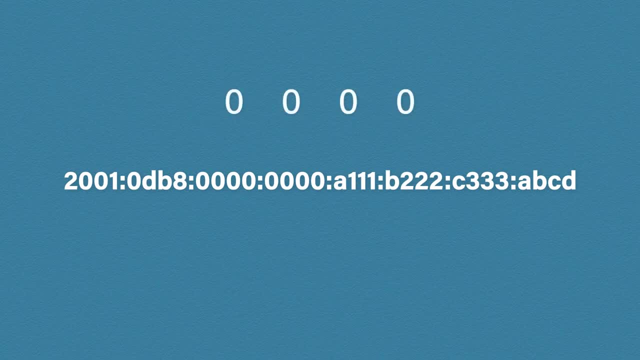 made up of four binary bits. These bits can either be a 0 or a 1.. Each bit represents a value of 1,, 2,, 4 or 8.. It doubles with each column from right to left. Wherever we see a 1, that toggles that. 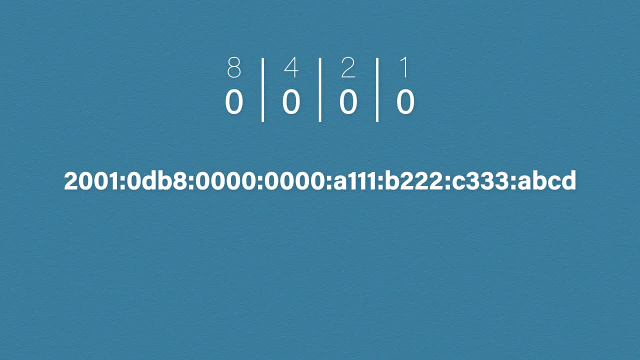 column on and wherever we see a 0 that toggles the column off. We then add up all of the columns that have a 1 and this gives us our number or letter. So let's take the first number from the address, which is 2.. How do you? 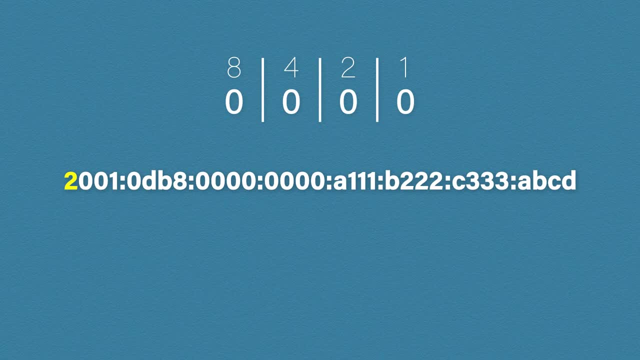 think we can make the number 2 from our binary bits. We simply add a 1 in the 2 column. All other columns stay a 0 because we don't need them. So the binary value for our first number is 0010.. We're going to go through a few of these. 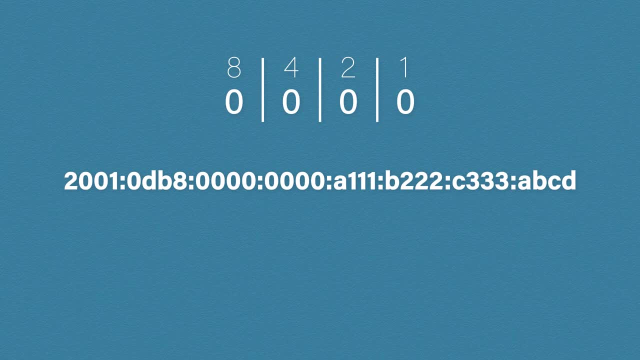 just to make sure it sticks. The second number in our address is 0. how do we get 0?? Well, we simply leave all the columns off, so this gives us a binary value of 0000.. Our next number is also 0, so it's the same. 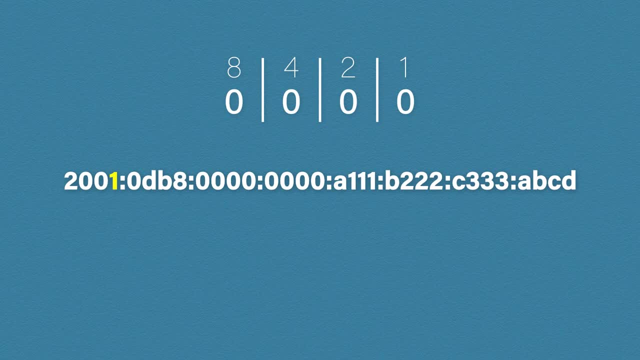 Now we have number 1.. Just like with before, we turn on the column for 1 and we leave the rest to 0.. Our binary value is 0001.. We have yet another zero, so we know our binary value will be: well, all zeros. This next one we do need. 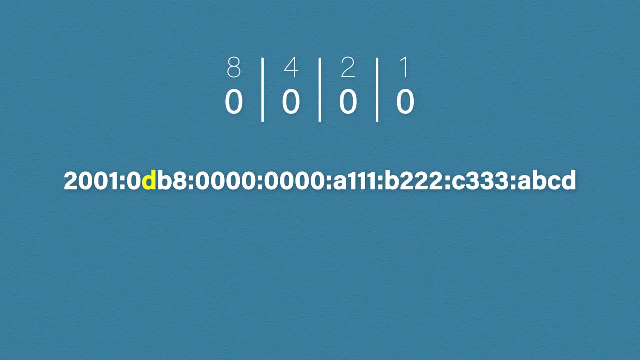 to look at. How do you think we get the letter D from our binary chart? Well, if you remember, I mentioned that each character can either be 0 to 9 or A to F. Clearly, we can make bigger numbers with our binary chart than 9.. In fact, we can. 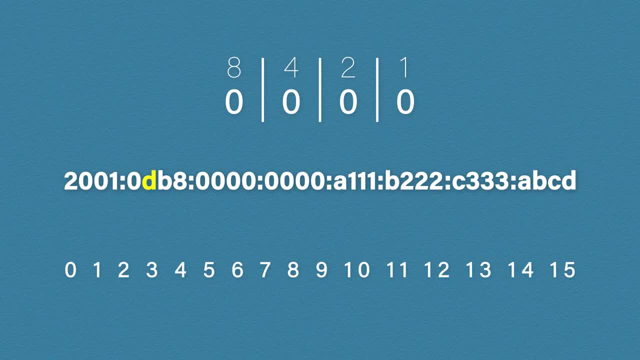 get up to the number 15 if we turn on all the columns with a 1.. The problem is we can't use double digits, so instead we swap out 10,, 11,, 12,, 13,, 14 and 15 for A B. 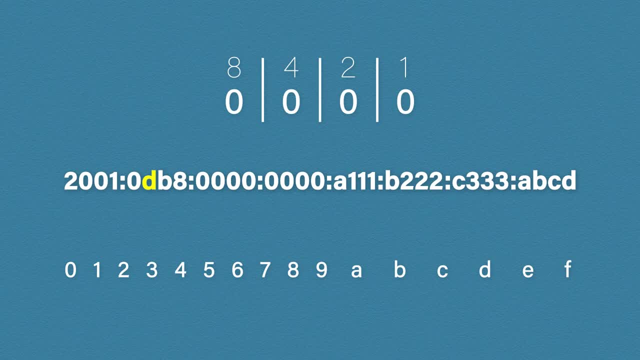 C, D, E and F. So now we know that. how do we get the letter D? D has replaced the value 13, so this is the number we need to get. You should always start with the highest number you can, and in this case, 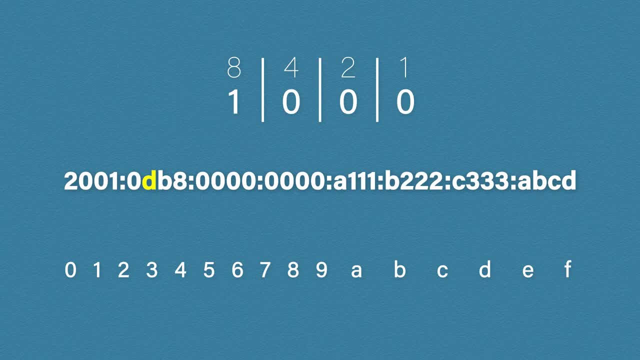 that number is 8.. Then the second highest, which is 4, this gives us 12, so we only need one more. We'll leave the 2 column off, because this would make our number too high, and turn on the 1 column. Add this all up and we get 13, so that 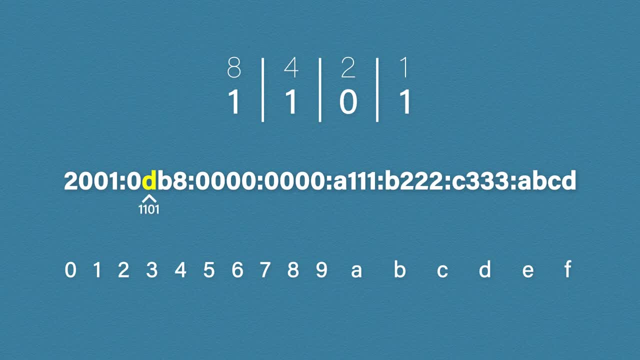 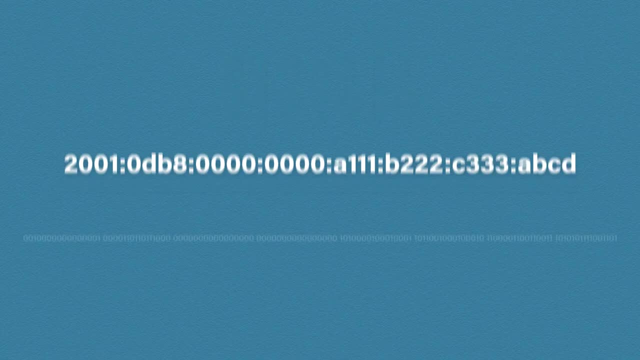 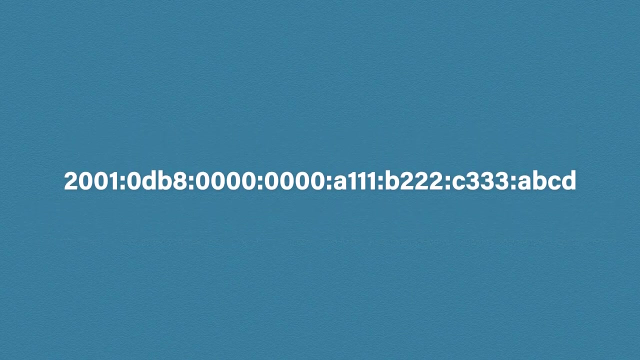 means our binary value for D is 1101.. Hopefully you get the idea by now. If you were to continue doing this, you would eventually end up with the full binary value. Okay, so that's our brief binary lesson. It's not something you'll do every day. 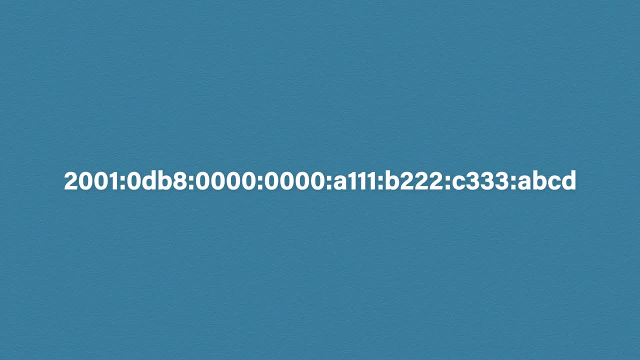 but it is important to understand, especially when looking at some more in-depth subnetting. Okay, so, just like IP version 4, IP version 6 has a network section and a host section. The way IPv4 does this is by using a subnet mask. 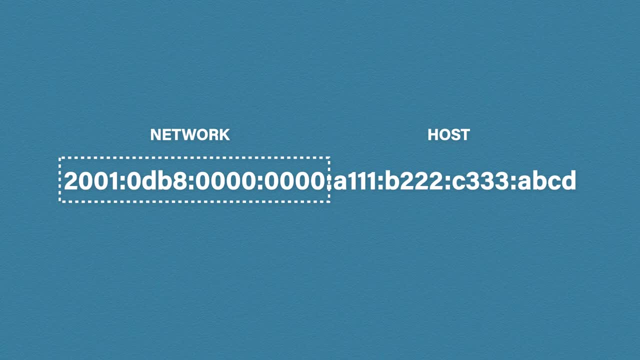 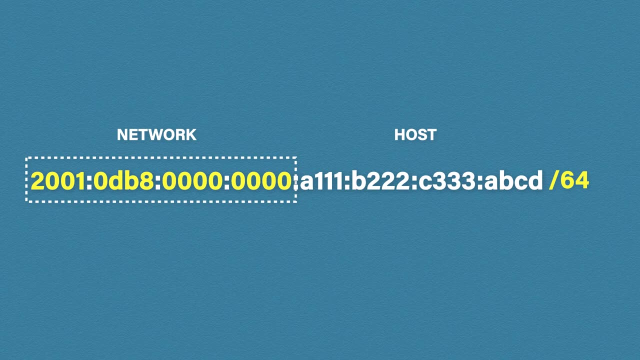 However, IP version 6 has gotten rid of the subnet mask and instead it just uses a forward slash and the number is changed. So that's the first step. Now let's try this of network bits, which you should be familiar with from IPv4.. So in our example, slash64 is half of 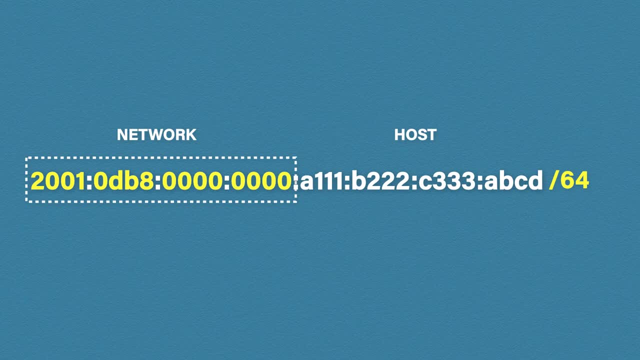 our 128-bit address. Slash64 addresses are common when it comes to IPv6.. It splits it nicely down the middle and ensures we have plenty of networks and plenty of hosts. but be prepared to see different numbers. Remember each character is 4 bits long. 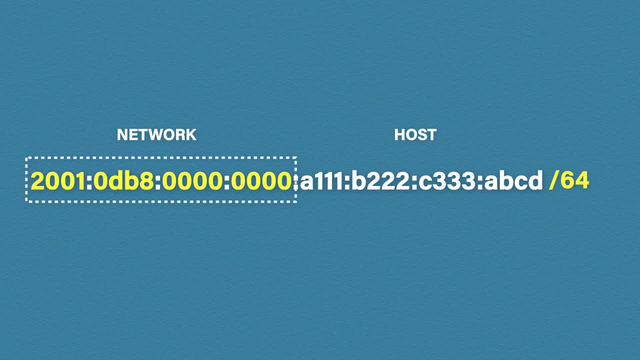 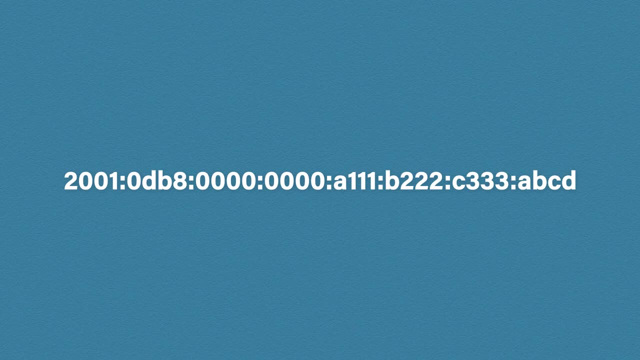 and each hextet is 16 bits. We'll now look at how we can press this address to make it look a little nicer. I'm sure we can all agree that this is a lengthy address and the thought of typing this out over and over again is simply horrific. But there are a couple. 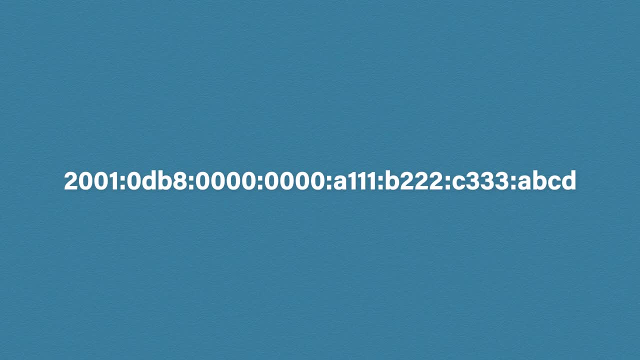 of tricks that we can do to make this address a bit more bearable. The first trick is to remove continuous zeros, Because we find ourselves with so many addresses a lot of the time we see more and more numbers. We can simply replace multiple hextets next to each other that contain: 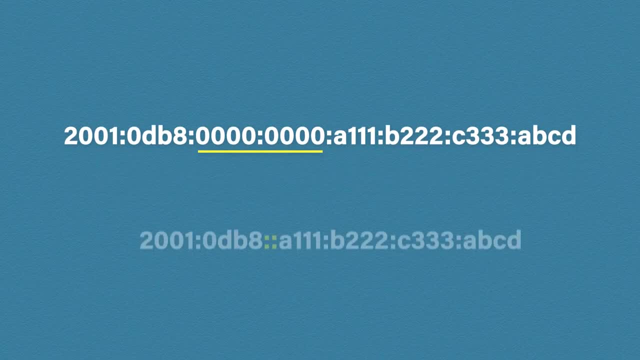 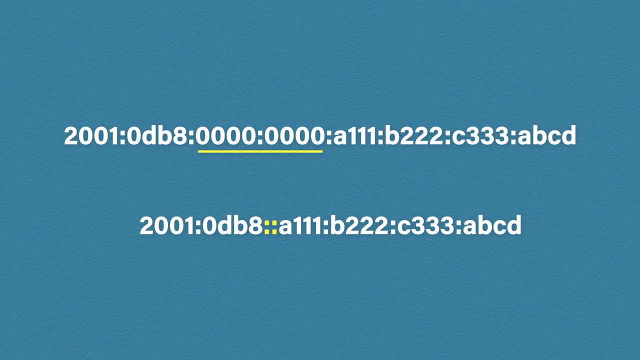 only zeros. We can simply replace all of these zeros with a double colon. When the computer sees this address, it sees the double colon, works out there are two missing hextets and then fills in the zeros. The rule to this trick is it can only appear once. For example, if we change this address slightly and 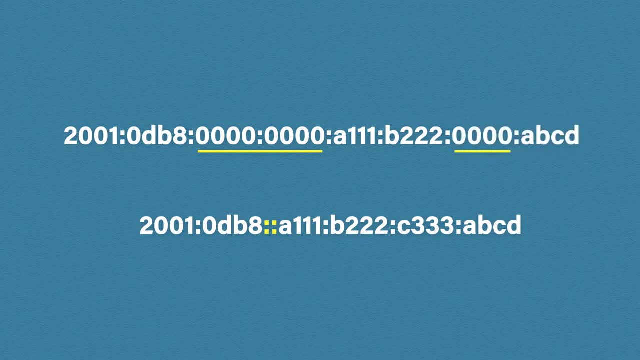 add another hextet of zeros. we cannot add another double colon. If a computer looked at this address, it has no way of filling in the missing pieces. How would it know if the address is missing eight zeros from here and four zeros from there, or four zeros? 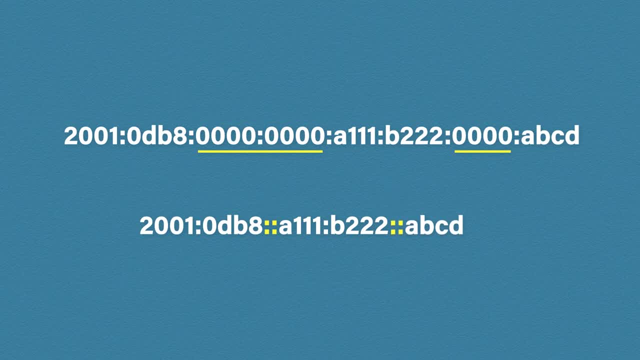 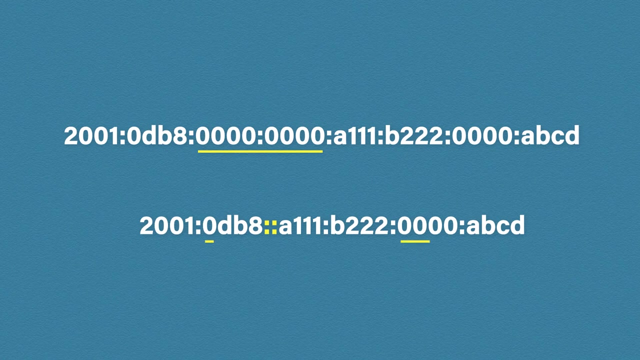 from here and eight zeros from there. So this is why it can only happen once. But there is another trick we can use. We take all of the leading zeros from each hextet to where it starts with one or more zeros. We have one here and three there. 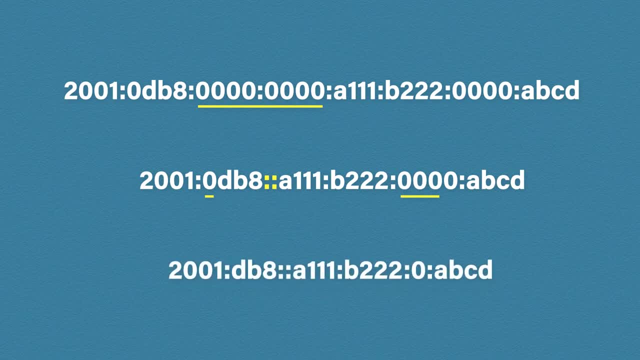 Then we simply remove them. So now, when the computer looks at db8, it realizes there is a missing character and it fills in the gap. The same thing happens on this hextet. Note that even though it's all zeros, because we already used the double colon, we need to leave the last zero. 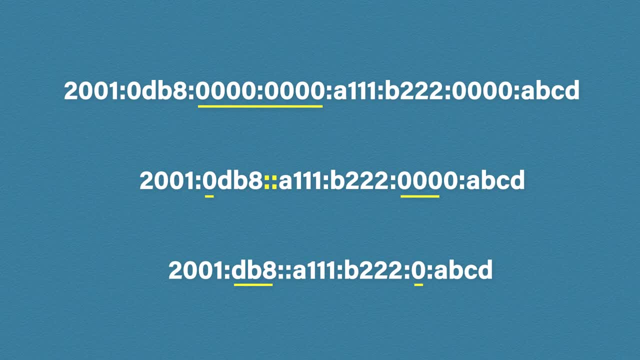 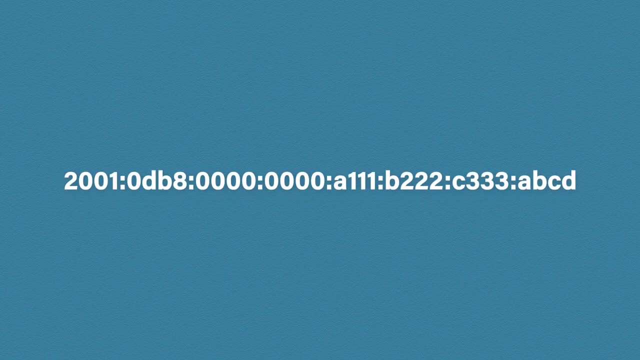 And this is the address we're left with, Still pretty large, but it's a big improvement from where we started. Okay, so moving on, Just like ipv4, there are different types of ipv6 addresses and they serve different purposes. What we see here is called a global unicast address. 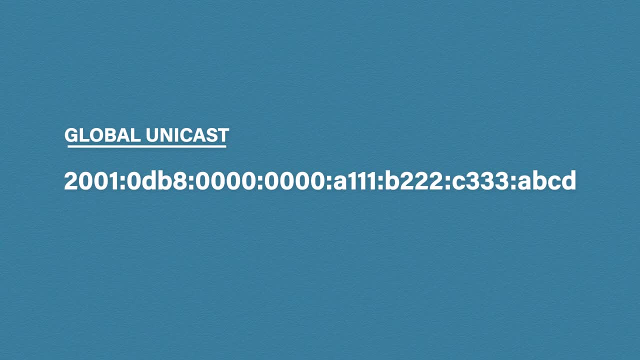 You can think of this like a public ipv4 address that is routable over the internet, Unlike ipv4. because we have such a massive amount of ip addresses, we no longer need to rely on private addresses. Every device can have its own public ip address. The first part of this address is known as a global prefix. 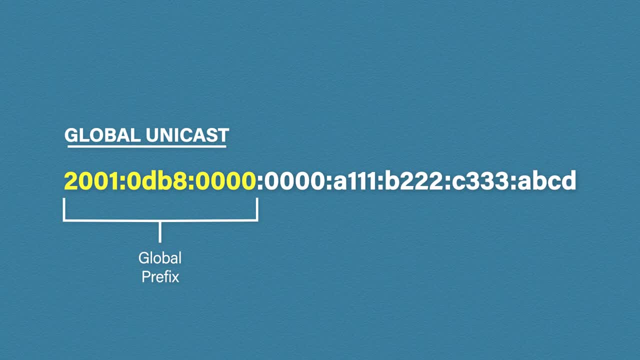 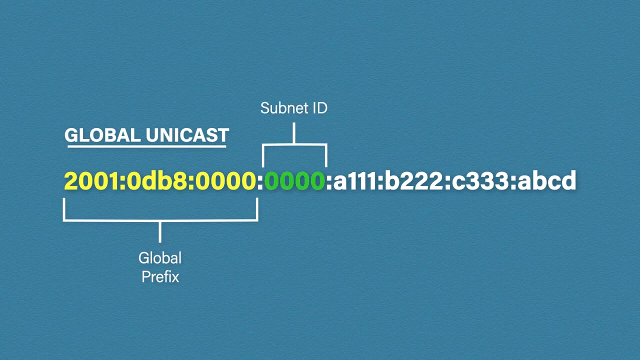 This is what your isp will provide you as a block of ip addresses. This global prefix will be a minimum of 48 bits long. Once we have the global prefix, we can then use the next 16 bits for our subnet id. 16 bits gives us over 65 000 subnets to. 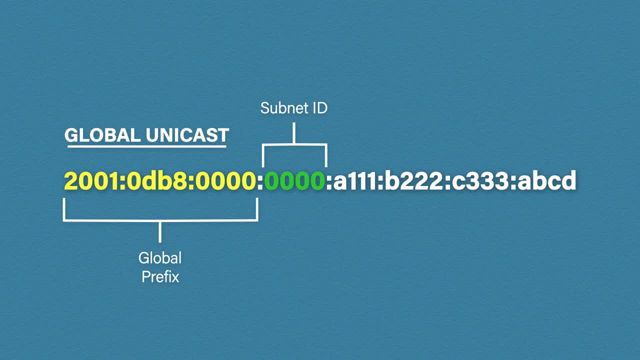 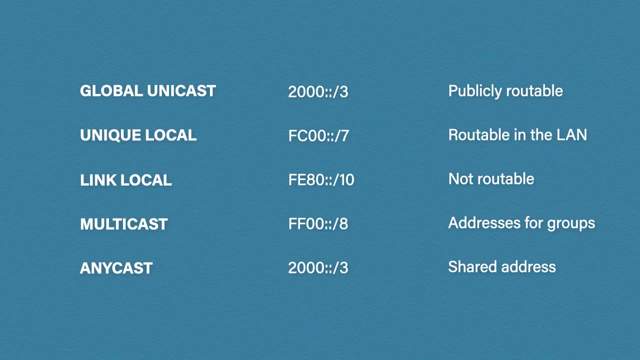 play with and that leaves us nicely with a 64-bit host or interface id. Okay, so let's look at some other address types. We have global unicast, which we just looked at. This is a publicly routable address, like the ip version for public ips, The prefix to identify these. 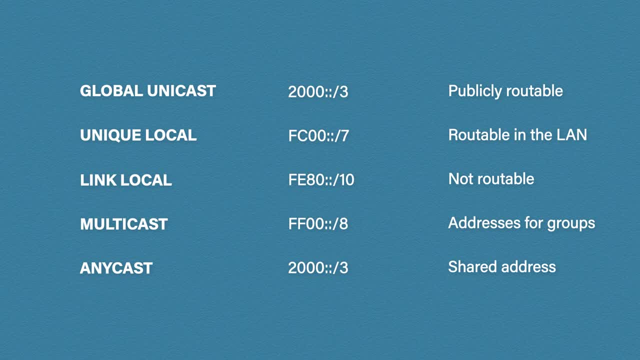 addresses is 2000, double colon slash three. This means the first three bits identify a global unicast address. It will start with either a two or a three. Next we have a unique local address. This address is like an ip version for private address. These are not globally routable. 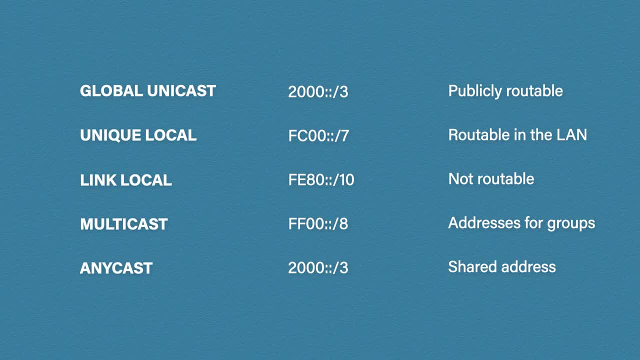 The prefix to identify a unique local address is fc, double zero, double colon slash seven. Using the first seven bits, a unique local address will always start with an f, followed by either a, c or a d Link local addresses. Think of these as quick, automatic private ip addresses that are: 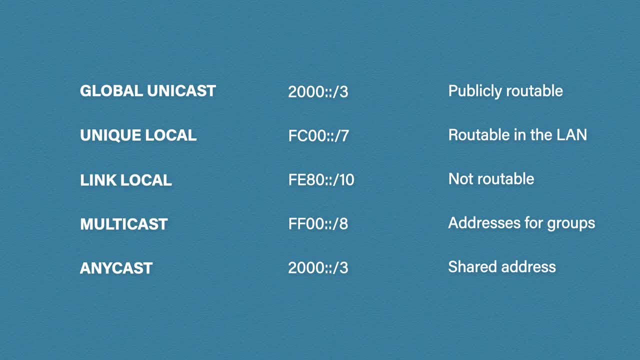 not routable over a network. They are designed to communicate only within a single area of a network. You may have seen the dreaded 169.254.. something dot, something address when your computer can't connect. This is pretty much the ip version 6. 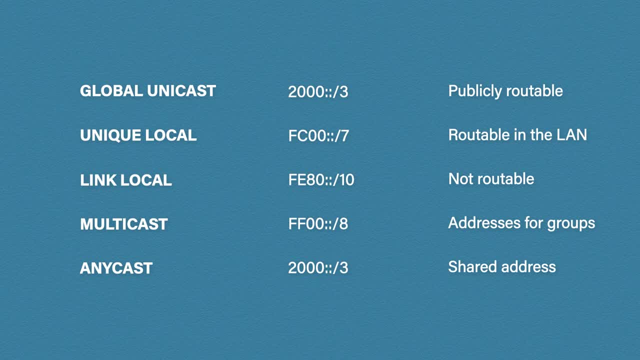 replacement. You can identify a link local address because it has a prefix of fe 80 colon, colon slash 10.. This means the link local address will always start with fe. Multicast addresses: These are addresses that are sent to a group of computers. 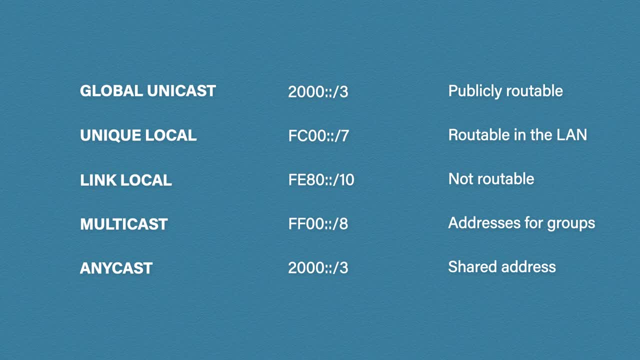 or devices listening for that particular multicast address. IP version 4 used to also use broadcast addresses. These were sent to all computers within a network. These have now been scrapped with ip version 6.. Multicast addresses are easy to spot because they always start. 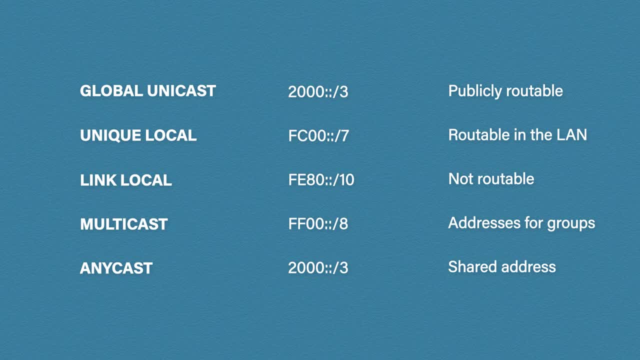 with f, f. Okay, last but not least, we have something called an anycast address. Now, these are interesting because ip version 6 allows us to assign the same ip address to multiple devices. The data is then sent to the closest device with that address. There isn't a specific ip range for anycast addresses.